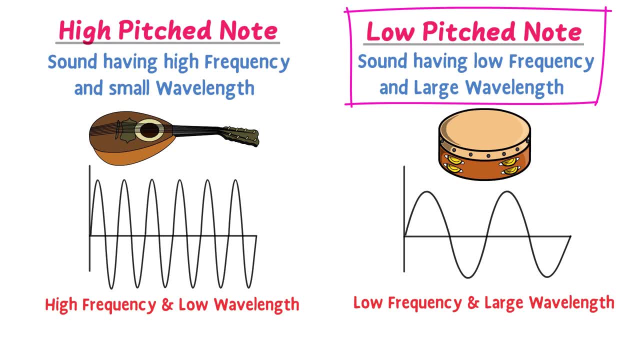 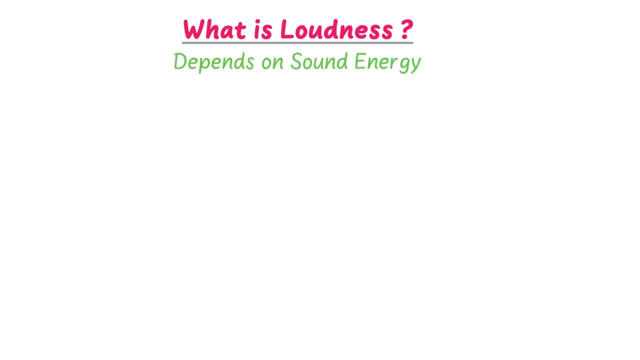 While low-pitched note has low frequency and large wavelength. Now, what is loudness? Well, loudness of a sound depends on sound energy. The greater is the sound energy, the larger is the loudness of a sound, and vice versa. 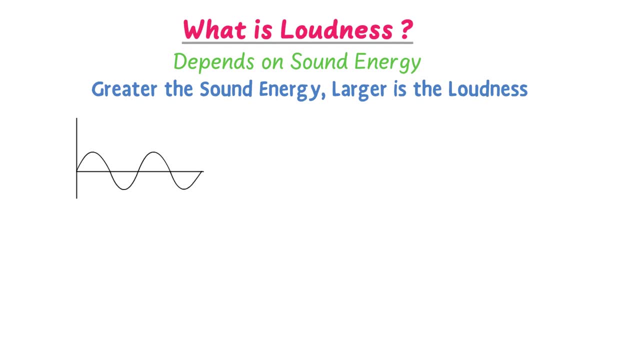 For example, consider this sound and this sound. This is a quiet sound and this is a louder sound. Now, why is this a quiet sound and this is a louder sound? It is because sound is small while the amplitude of this sound is large. So this is a quiet sound and this is a 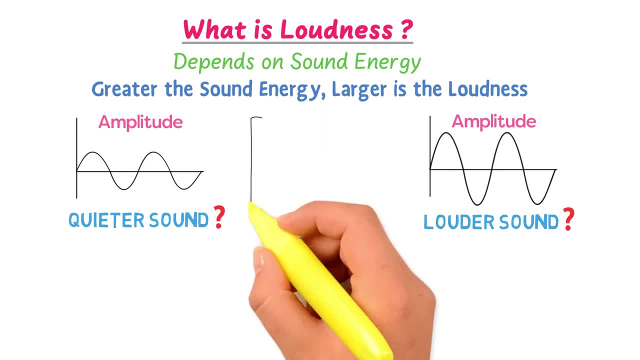 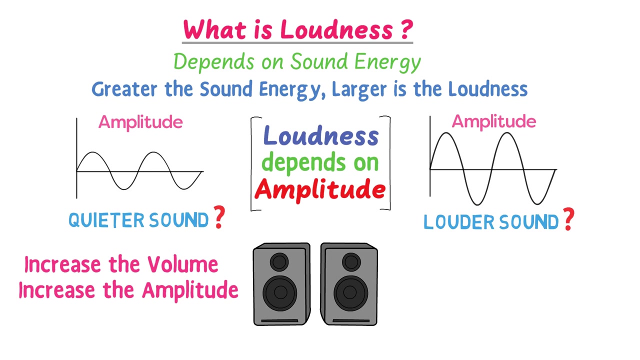 loud sound. Also noted down, this important MCQs: loudness of a sound depends on amplitude. Let me repeat it: Loudness of a sound depends on amplitude. For instance, when you increase the volume, the speaker increases the amplitude of the sound and you listen loud music. In contrast, 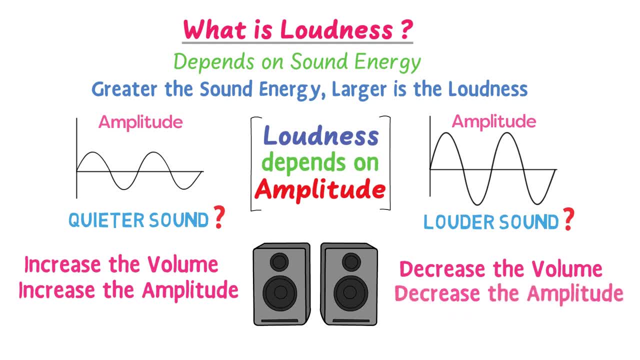 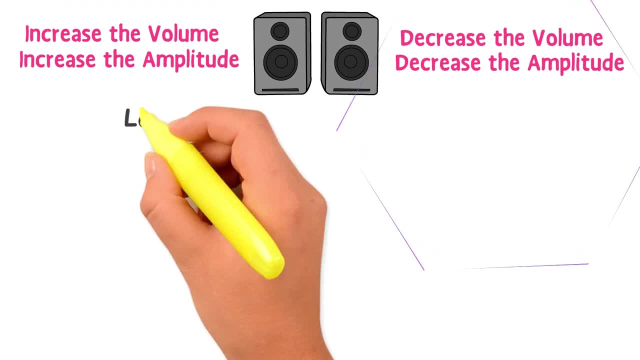 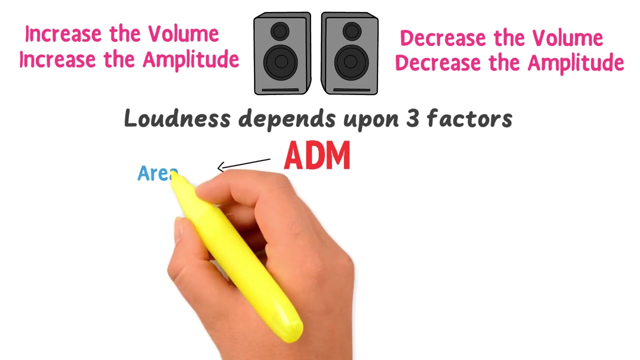 when you decrease the volume, the speaker decreases the amplitude of the sound and you listen quiet or low music. Remember that loudness depends upon three factors. My personal mnemonic, which I usually teach to my students, is Adam. to remember these three factors Here: A stands for area of vibrating or oscillating object. D stands for distance from a source. 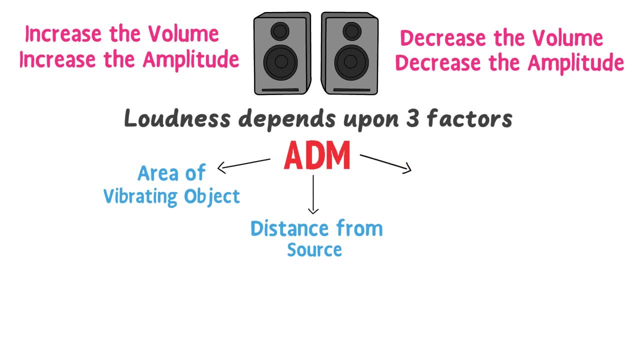 producing sound, And M stands for medium through which sound travels. Now consider a small doll and a big doll. Small doll produces low sound or quiet sound, and big doll produces loud sound or high sound, Because the vibrating area of this doll is small and the vibrating area of this doll is large. This 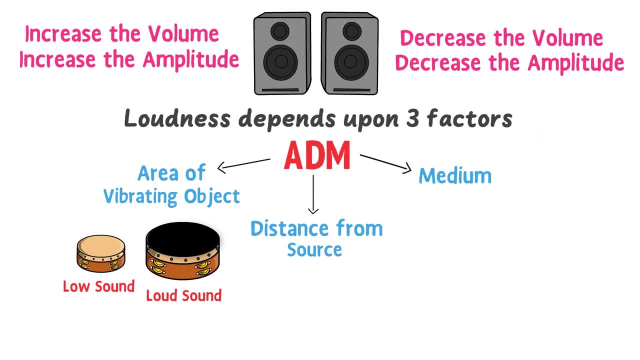 large vibrating area produces loud sounds and vice versa. Secondly, distance from a source of a sound means if you stand near the source, you listen loud sound. If you stand or move away from the source, you listen quiet or low sound. And M stands for distance from a source And M stands for 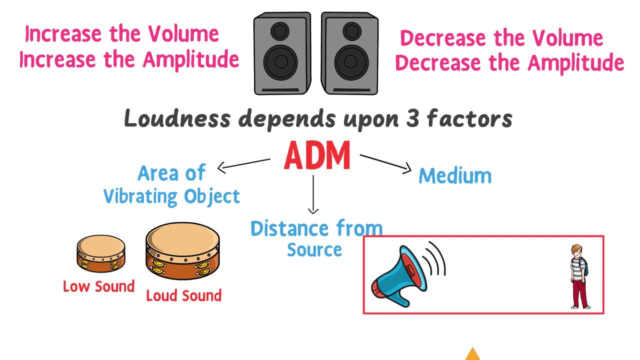 sound. Thus increasing the distance from a source means decreasing the loudness. Thirdly, medium in which sound travels means the speed of a sound is maximum and solids, then in liquids and then in gases. Same sounds have different loudness and different media. So therefore, 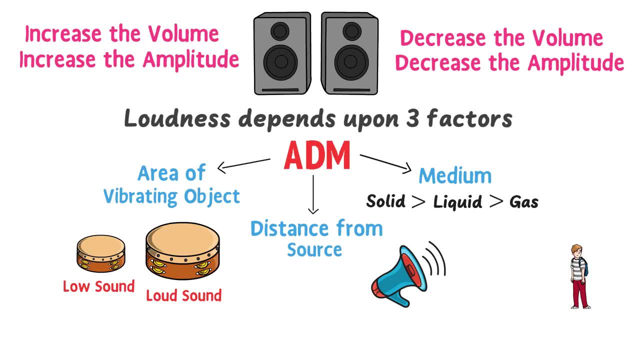 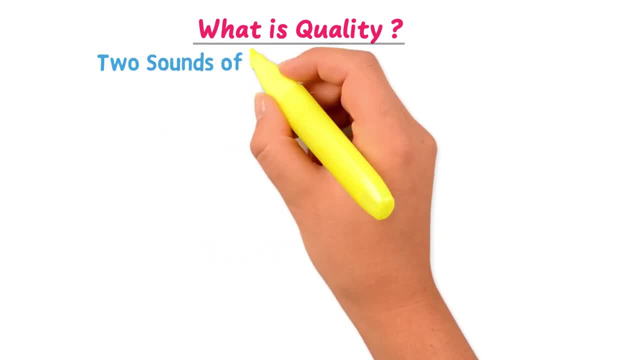 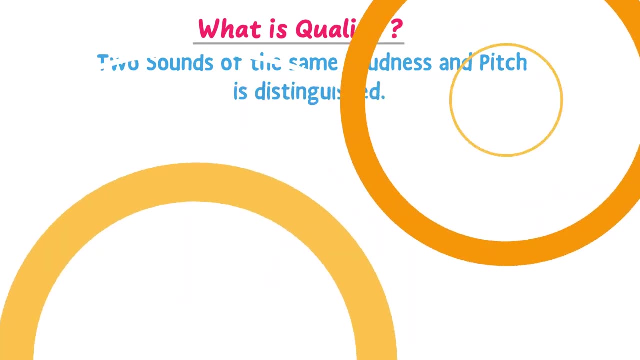 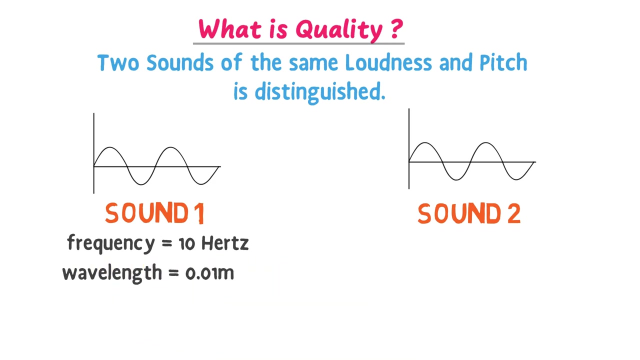 remember this mnemonic Adam Supporting sounds in crawls, making a sound and another sound are used, or sounds of softness, as well as contrasting quarterback sounds. There are two crispy horns in one of these sounds, One good sound and another one not terribly. good sounds. The first sound of the sound in the second sound will result in softness and no 해도an troh میں sound of noise. or The third sound of sound will result in high sounds. And the fourth sound of the sound is the property of sound. It is the property of a sound by which two sounds of the same share is very much distinguishable. 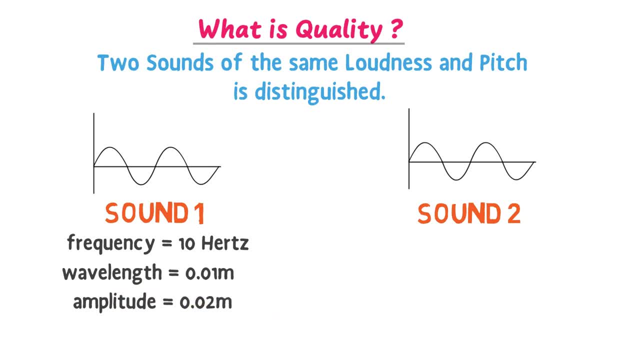 is equal to 0.02 meter. Also, this sound 2 has frequency f is equal to 10 hertz, wavelength is equal to 0.01 meter and amplitude is equal to 0.02 meter. It means that these both sounds have. 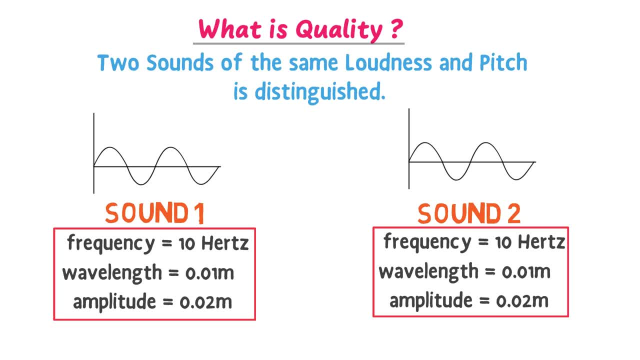 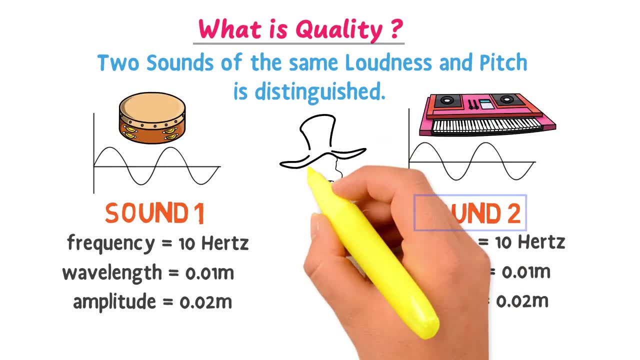 same frequency, same wavelength and same amplitude. Now I play sound 1 on a doll and sound 2 on a piano. Can you differentiate between sound 1 and sound 2?? Well, the answer is yes. You say sound 1 is the sound of a doll and sound 2 is the sound of a piano. So you differentiate them due to. 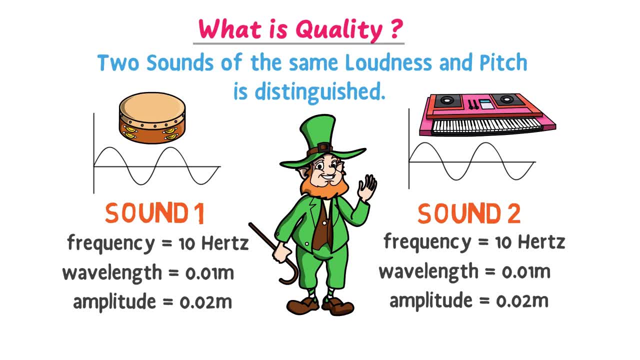 quality of a sound. Therefore, we say that quality of a sound distinguishes two sounds of the same loudness and pitch if they are played on different instruments. This was all about pitch, loudness and quality of a sound.